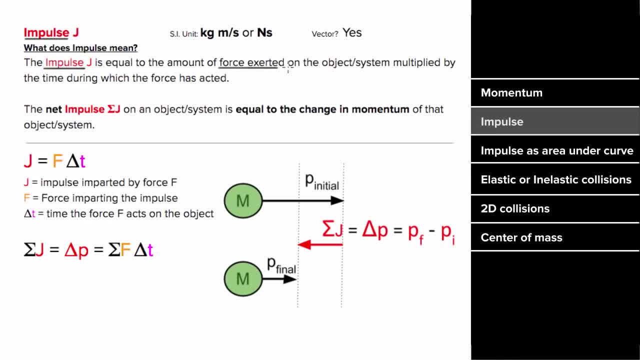 What does impulse mean? The impulse is the amount of force exerted on an object or system multiplied by the time during which that force was acting. So in equation form that means that J the impulse is equal to the force multiplied by. 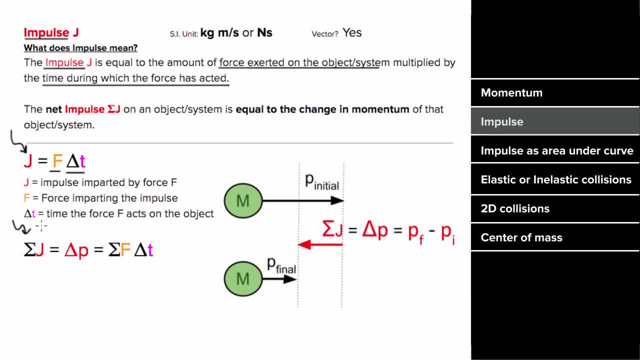 how long that force was acting, And the net impulse is gonna be equal to the net force times the time during which that net force was acting. And this is also gonna be equal to the change in momentum of that system or object. In other words, if a mass had some initial momentum, 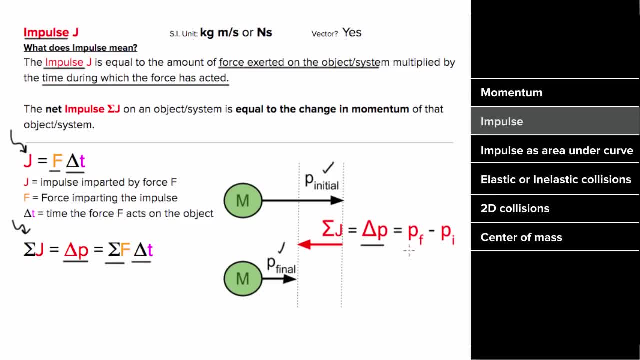 and ends with some final momentum. the change in momentum of that mass- P final minus P initial- is gonna equal the net impulse, And that net impulse is gonna equal the net force on that object multiplied by the time during which that force was acting. 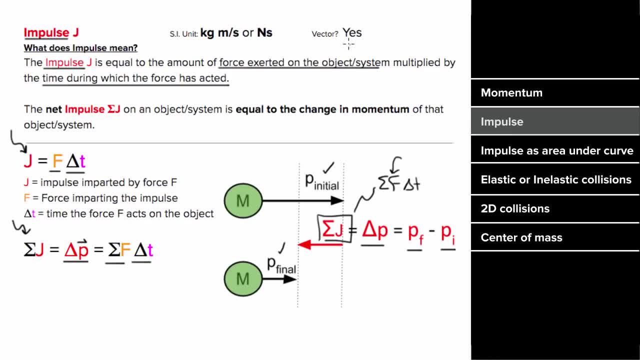 And since impulse is a change in momentum and momentum is a vector, that means impulse is also a vector, So it can be positive and negative And the units are the same as momentum, which is kilograms times meters per second. Or, since it's also force, times time. 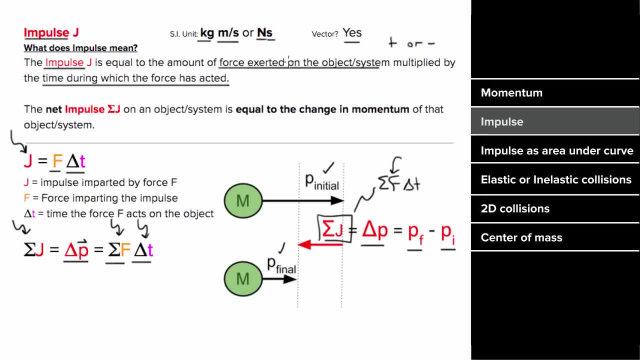 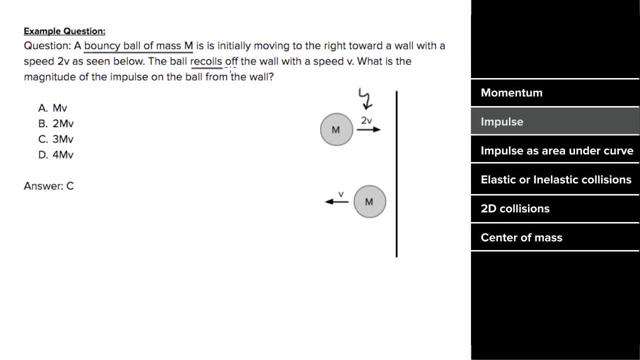 you could write the units as newtons, times, seconds. So what's an example problem involving? what does an impulse look like? Let's say, a bouncy ball of mass M is initially moving to the right with a speed two V And it recoils off a wall with a speed V. 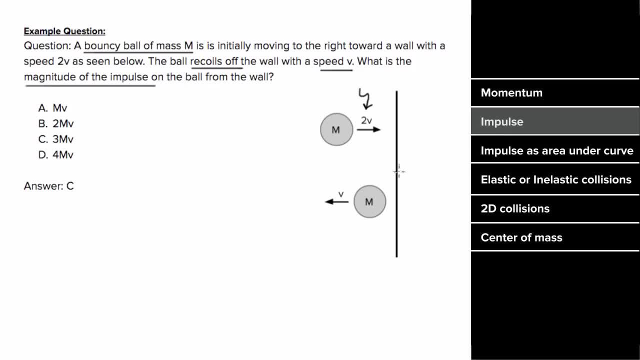 And we wanna know what's the magnitude of the impulse on the ball from the wall. So the impulse J is gonna be equal to the change in momentum. The change in momentum is P final minus P initial, So the final momentum is gonna be the mass. 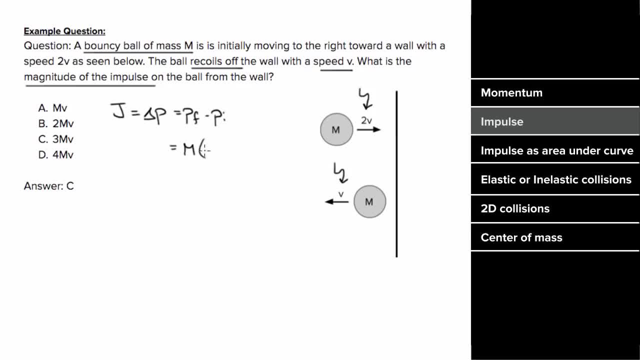 times the final velocity, but this velocity's heading leftward. so you can't forget the negative sign. minus the initial momentum, which would be M times two V, which gives a net impulse of two V, The net impulse of negative three M V. 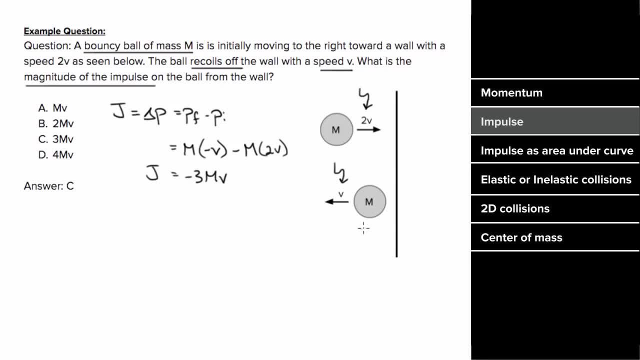 and this makes sense. the net impulse has to point in the same direction as the net force. This wall exerted a force to the left. That means the impulse also points left and has a magnitude of three M V If you get a force versus time graph. 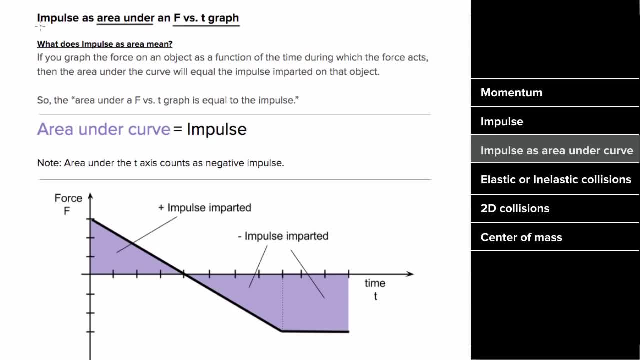 the first thing you should think about is that the area under that graph is gonna equal the impulse on the object. So if you graph the force on some object as a function of time, the area under that curve is equal to the impulse. Just be careful, since area above this time axis. 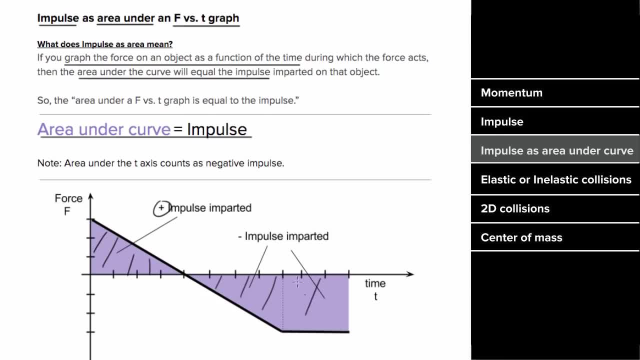 is gonna count as positive impulse and area underneath the time axis would count as negative impulse, since those forces would be negative. Why do we care that the area is equal to the impulse? Well, if we can find the area that would equal the impulse. 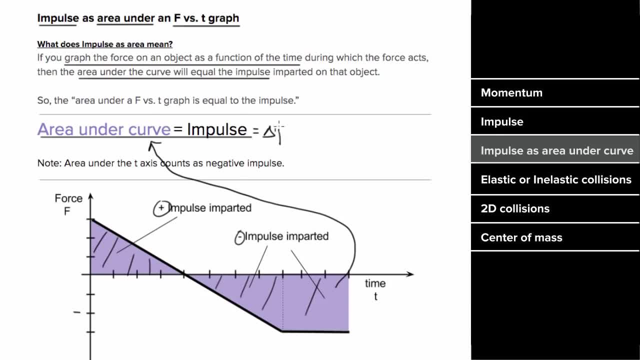 and if that's the net impulse on an object, that would also equal the change in momentum of that object, which means we could figure out the change in velocity of an object. So what's an example problem involving impulse as the area under a graph look like? 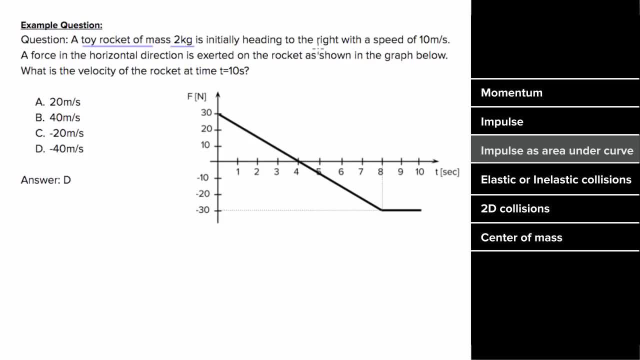 Let's say, a toy rocket of mass two kilograms was initially heading to the right with a speed of 10 meters per second and a force in the horizontal direction is exerted on the rocket as shown in this graph. and we wanna know what's the velocity of the rocket. 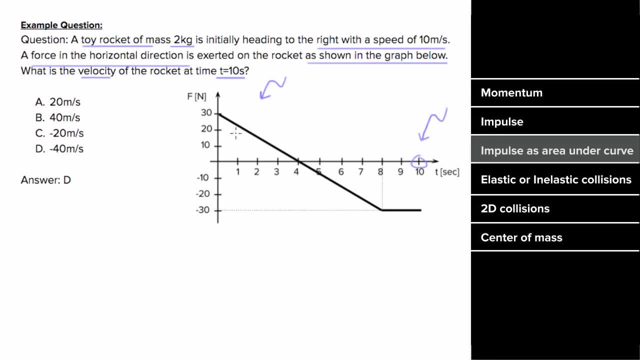 at the time. t equals 10 seconds. To figure that out, we'll figure out the area under the curve. This triangle would count as positive area, This triangle would count as negative area and since this triangle is just as positive as this triangle is negative, 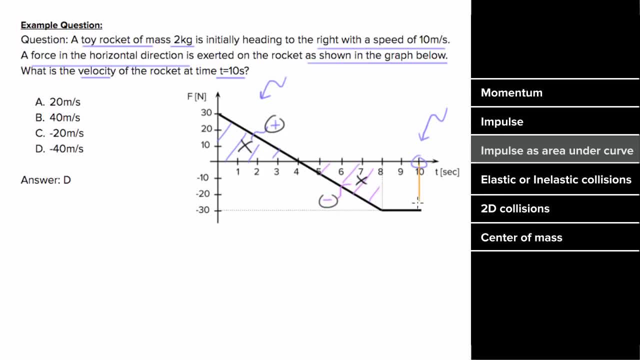 these areas cancel completely, and the only area we'd have to worry about is the area between eight seconds and 10 seconds. This is gonna end up being a negative area, since the height of the rectangle is negative 30, and the width of the rectangle is gonna be two seconds. 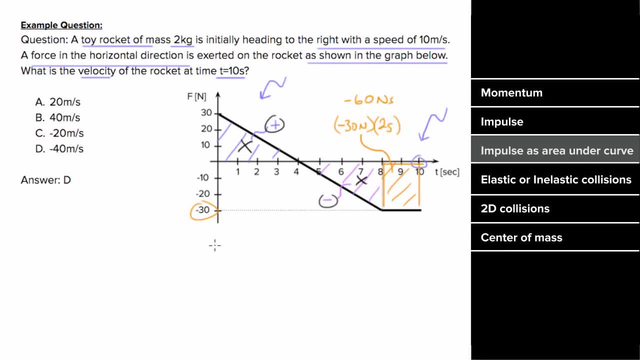 This gives an impulse of negative 60 Newton seconds. So if the impulse on this object is negative 60 Newton seconds, that's gonna equal the change in momentum of that object. How much momentum did this object start with? The initial momentum of this object? 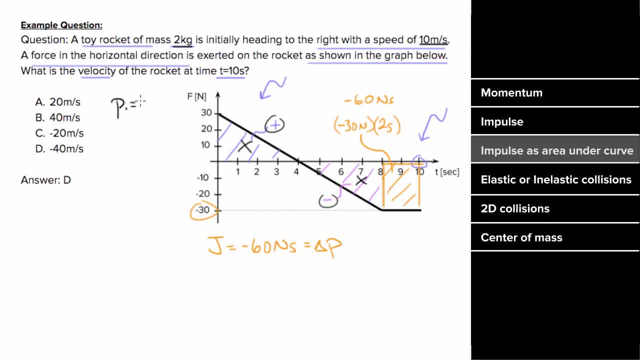 is gonna be two kilograms times the initial velocity, which was 10 meters per second to the right, which is positive 20 kilogram meters per second. So if the initial momentum of the rocket is positive 20, and there was a change in momentum of negative 60,, 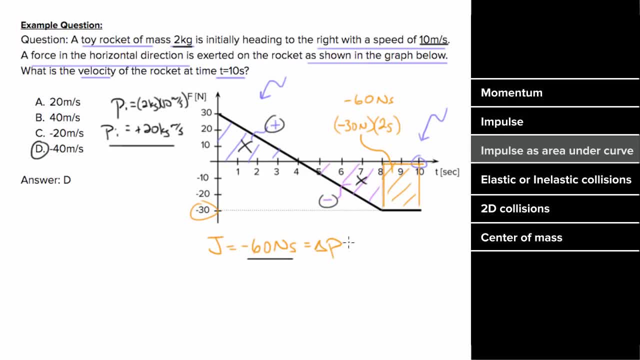 the final momentum just has to be negative 40. Or, in other words, since the change in momentum would have to be the final momentum minus the initial momentum, which was positive 20,, we could find the final momentum by adding 20 to both sides. 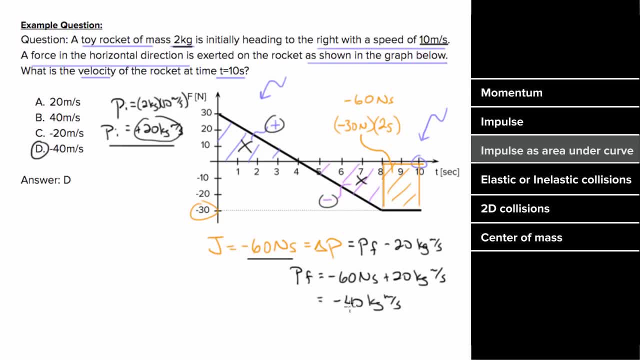 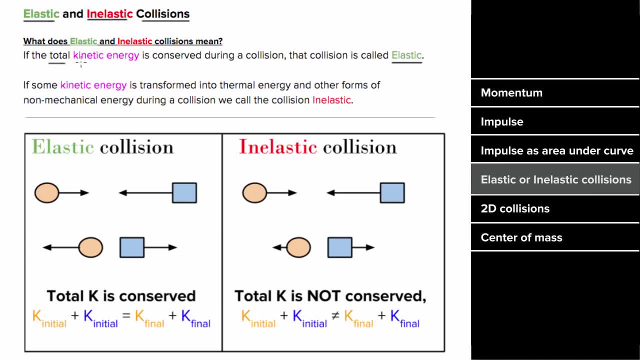 which would give us negative 60, plus 20,, which is negative 40.. What's the difference between an elastic and an inelastic collision? What we mean by an elastic collision is that the total kinetic energy of that system is conserved during the collision. 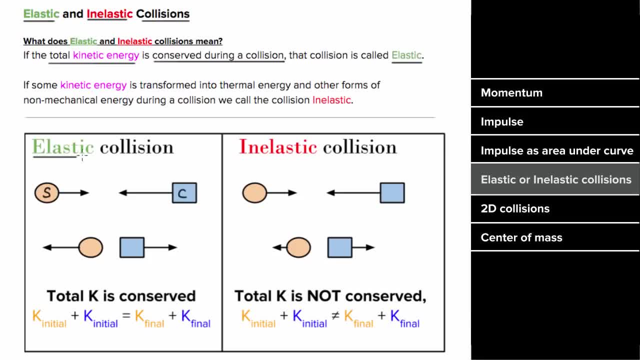 In other words, if a sphere and a cube collide, for that collision to be elastic, the total kinetic energy of the sphere plus the kinetic energy of the cube before the collision would have to equal the kinetic energy of the sphere plus the kinetic energy of the cube after the collision. 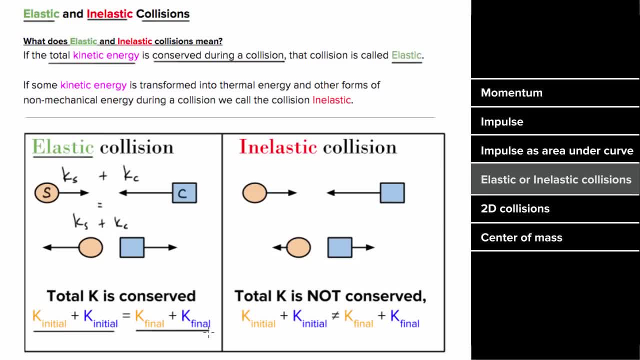 If the total kinetic energy before the collision is equal to the total kinetic energy after the collision, then that collision is elastic. It's not enough for the system to just bounce off of each other. If two objects bounce, the total kinetic energy might not be conserved. 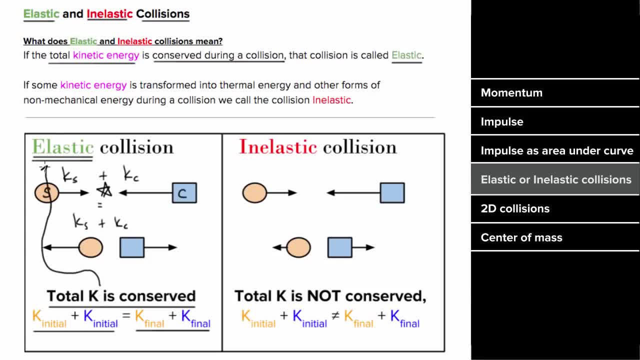 Only when the total kinetic energy is conserved can you say the collision is elastic. For an inelastic collision, the kinetic energy is not conserved during the collision. In other words, the total initial kinetic energy of the sphere plus cube would not equal the total final kinetic energy. 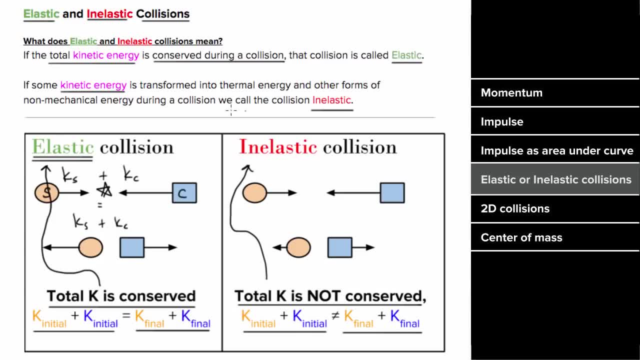 of the sphere plus cube. Where does this kinetic energy go? Typically, in an inelastic collision. some of that kinetic energy is transformed into thermal energy during the collision, While masses could bounce during an inelastic collision if they stick together. the collision is typically called 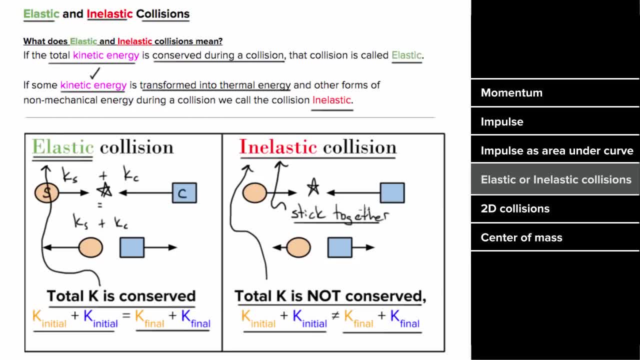 a perfectly inelastic collision, Since in this collision you'll transform the most kinetic energy into thermal energy, And when two objects stick together, it's a surefire sign that that collision is definitely inelastic. So what's an example? problem that involves 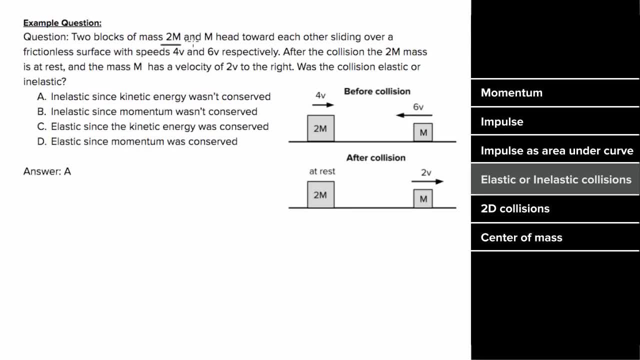 elastic and inelastic collisions look like, Let's say, two blocks of mass- 2m and m- head toward each other with speeds 4v and 6v respectively. After they collide, the 2m mass is at rest and the mass m has a velocity of 2v to the right. 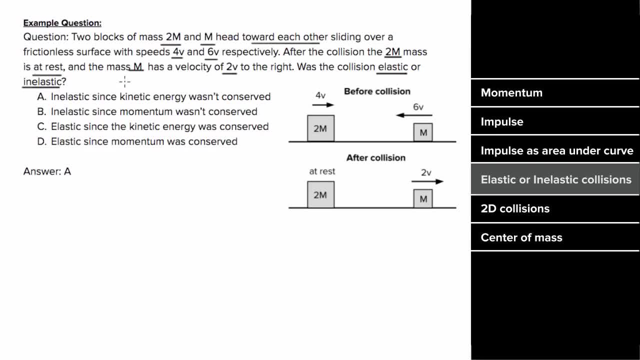 And we wanna know: was this collision elastic or inelastic? Now you might wanna say that since these objects bounced off of each other, the collision has to be elastic, but that's not true. If the collision is elastic, then the objects must bounce. 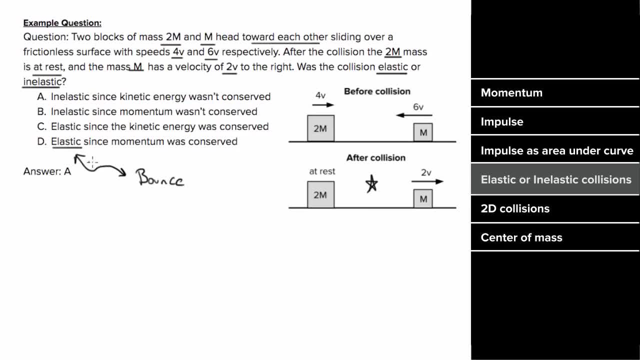 But just because the objects bounce does not mean the collision is elastic. In other words, bouncing is a necessary condition for the collision to be elastic, but it isn't sufficient. If you really wanna know whether a collision was elastic, you have to determine whether the total kinetic energy 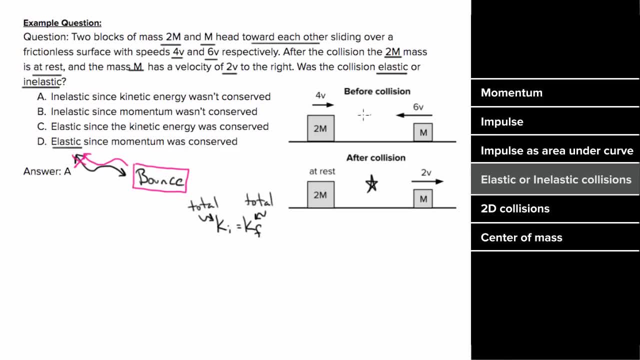 was conserved or not, And we can figure that out for this collision without even calculating anything. Since the speed of the 2m mass decreased, the kinetic energy of the 2m mass went down, And since the speed of the m mass also decreased, 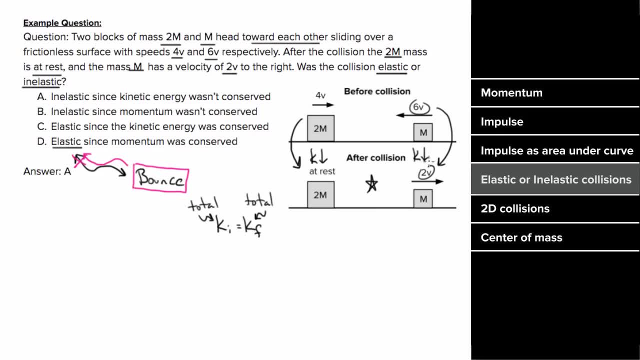 after the collision the kinetic energy of the mass m went down as well. So if the kinetic energy of both masses go down, then the final kinetic energy after the collision has to be less than the initial kinetic energy, which means kinetic energy was not conserved. 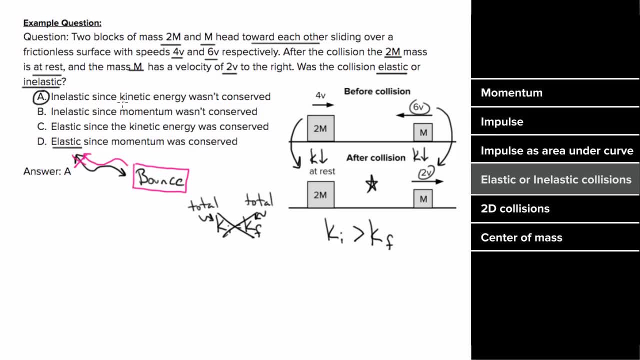 and this collision had to be inelastic. One final note: even though kinetic energy wasn't conserved during this process, the momentum was conserved. the momentum will be conserved for both elastic and inelastic collisions. It's just kinetic energy that's not conserved. 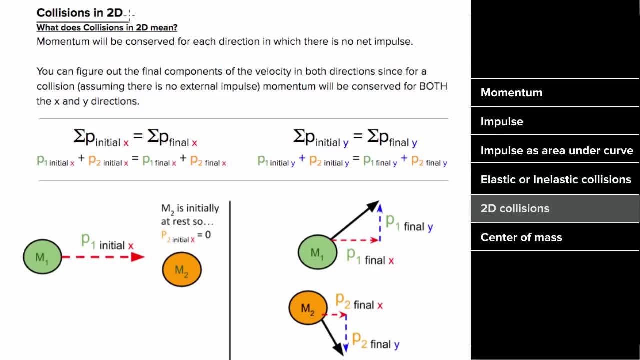 for an inelastic collision. How do you deal with collisions in two dimensions? Well, the momentum will be conserved for each direction in which there's no net impulse. If there's no net impulse in both directions, then the momentum in both directions. 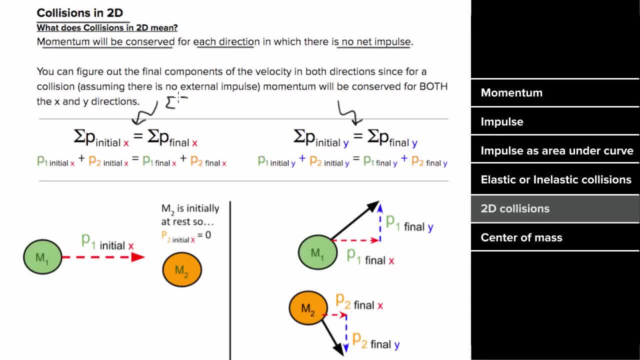 will be conserved independently. In other words, if there's no net force in the x direction, the total x momentum has to be constant, And if there's no net force in the y direction, the total momentum in the y direction has to be constant. 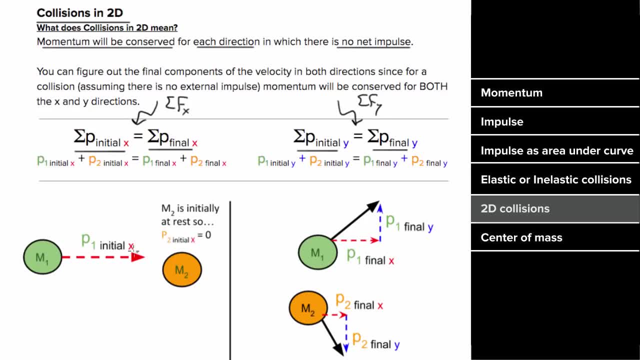 So in other words, if two spheres collide in a glancing collision, the total momentum in the x direction initially should equal the total momentum in the x direction finally, if there's no net impulse in that x direction, And the total momentum in the y direction initially. 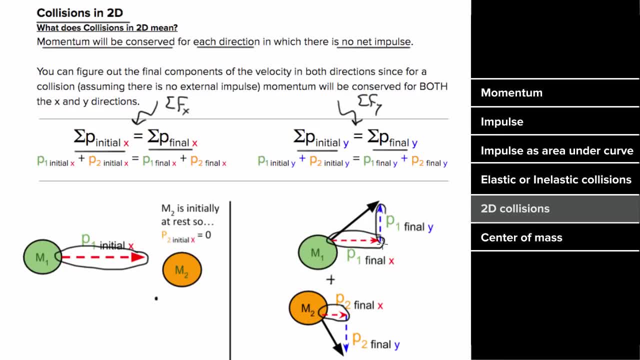 of which there is none in this case, would have to equal the total momentum in the y direction. finally, if there's no net impulse in the y direction. So what's an example involving collisions in two dimensions? look like, Let's say, a metal sphere of mass m. 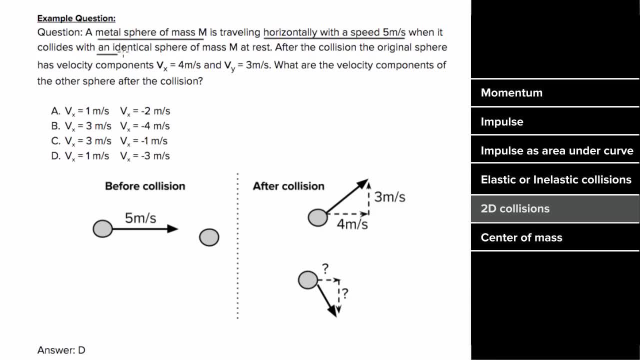 is traveling horizontally with five meters per second when it collides with an identical sphere of mass m that was at rest After the collision. the original sphere has velocity components of four meters per second and three meters per second in the x and y directions. 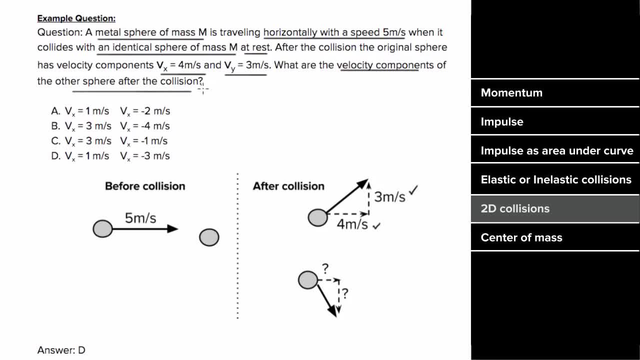 And we want to know what are the velocity components of the other sphere right after the collision. So, assuming there were no net forces in the x or y direction in this case, then the momentum will be conserved for each direction And since the mass of each sphere is the same, 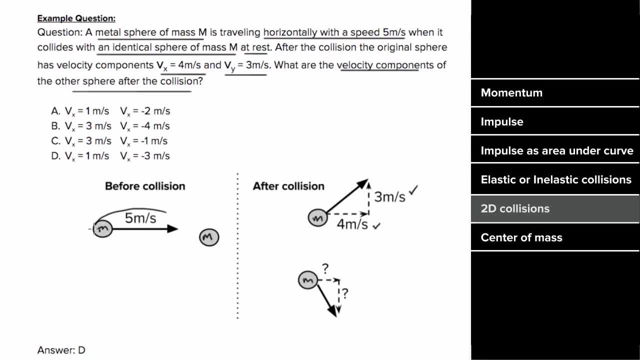 we can simply look at the velocity components. So if we started with five units of momentum in the x direction, we have to end with five units of momentum in the x direction. So the x component of the second sphere has to be one meter per second. 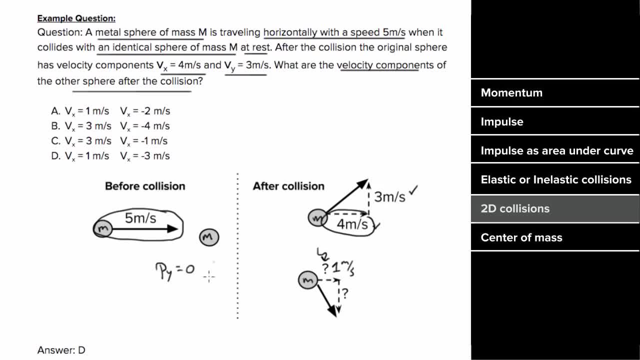 And since we started with no momentum in the vertical direction initially, we have to end with no momentum vertically. So if the first sphere has three units of momentum vertically after the collision, then the second sphere has to have three units of momentum vertically downward after the collision. 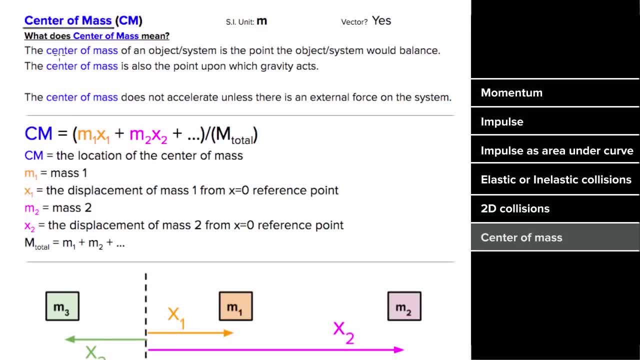 which gives us an answer of d. What's the center of mass mean? The center of mass of an object or a system is the point where that object or system would balance, And the center of mass is also the point where you can treat the entire force of gravity as acting. 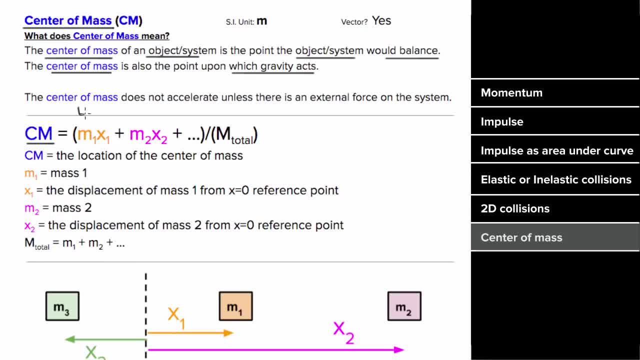 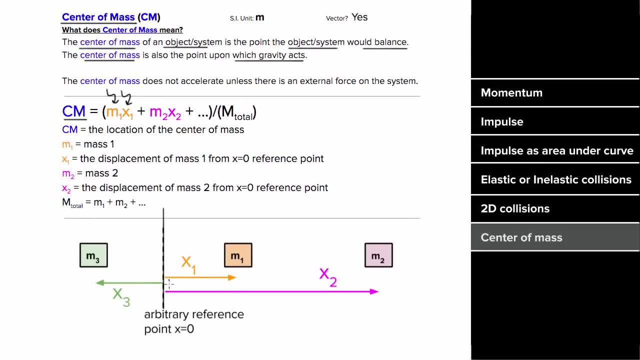 The way you can solve for the center of mass is by using this formula: You multiply each mass by how far that mass is from the reference point. If there's no reference point specified, you get to choose the arbitrary reference point which would designate where x equals zero. 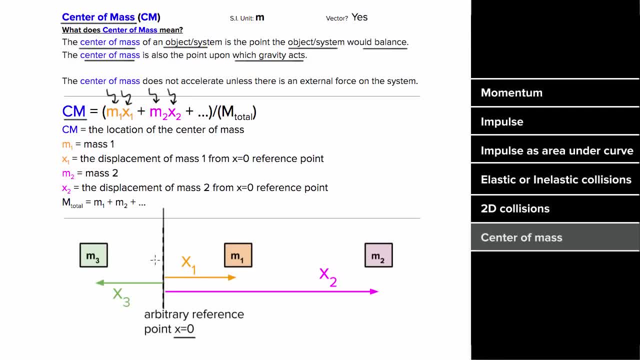 You continue adding each mass times its position. For positions to the left of the reference point, those would count as negative positions And when you're done accounting for every mass in your system, you divide by the total mass, which would be all the masses added up. 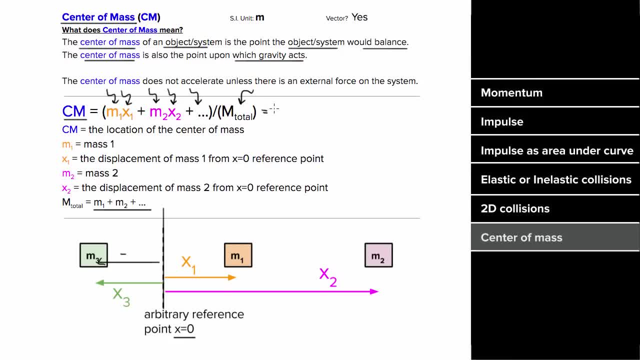 And the number you get would be the position of the center of mass. The center of mass is gonna have units of meters, since it's a location, The location where the system or object would balance and the location where you can treat the entire force of gravity as acting. 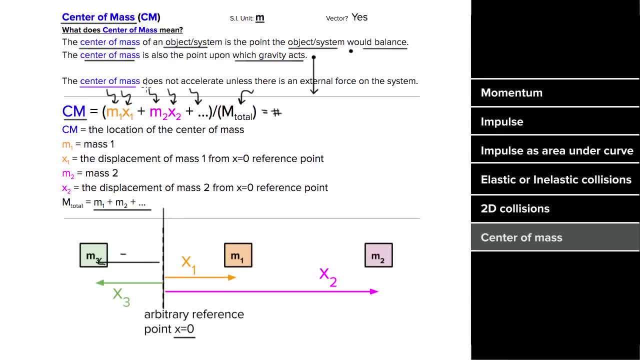 Something else that's extremely important to remember is that the center of mass of a system will not accelerate unless there's an external force on that system. In other words, the center of mass of a system follows Newton's first law. If the center of mass of a system is at rest, 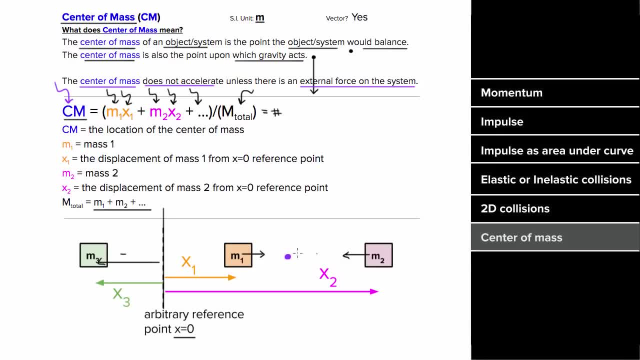 even if the masses in that system exert forces on each other and move around, the center of mass of that system will stay put until there's a net external force on the system And if the center of mass was initially moving to the right at some speed. 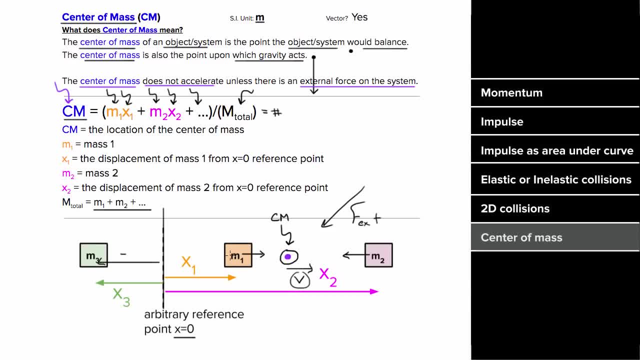 that center of mass will continue moving to the right at that speed, even if the masses are moving in different directions, until there's a net force on that system. So what's an example problem involving center of mass? look like, Let's say, a remote control car of mass m. 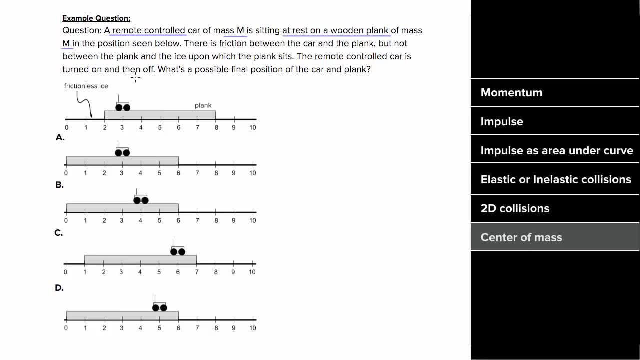 is sitting at rest on a wooden plank, also of mass m, and the center of mass of the system is at rest. So what's the position seen here? There is friction between the wheels of the car and the plank, but there's no friction between the plank and the ice. 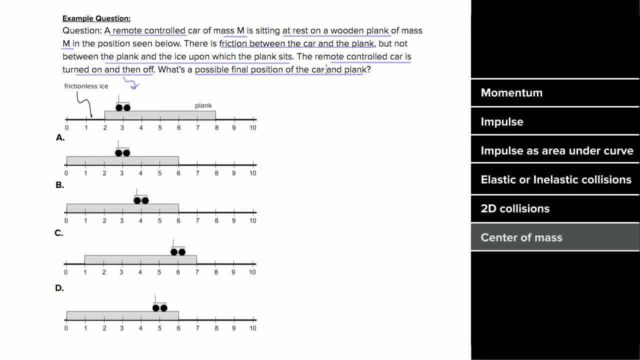 upon which the plank is sitting. Now the remote control car is turned on and off. What would be a possible final position of the car and the plank? Now? because the car is at rest and the plank is at rest, that means the center of mass of the system is also at rest. 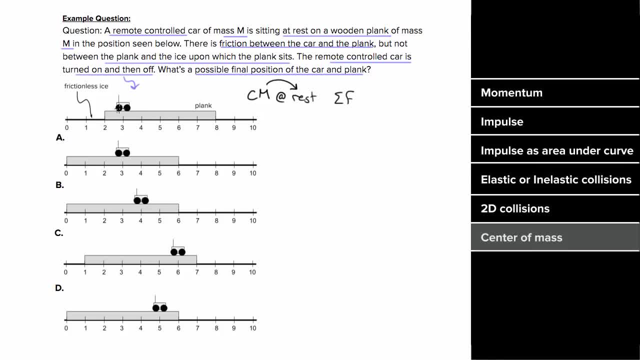 And since there's no net force on the system, the center of mass is going to have to remain at rest. Where is the center of mass? The plank's center is at five, so the center of mass between the car and the plank would be at the location of four. 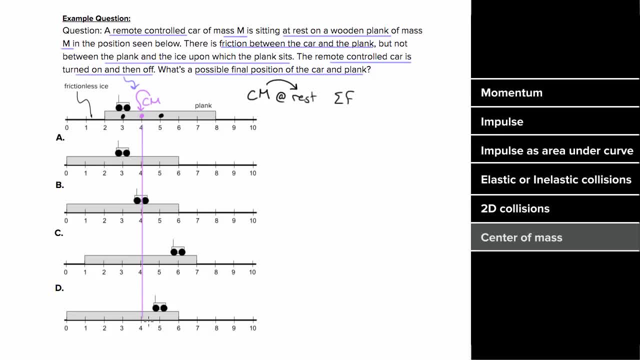 So to find the correct solution, we just need to figure out which one of these also has the center of mass at four. Option A has the car at three and the center of the plank at three. That'd put the center of mass at three meters.